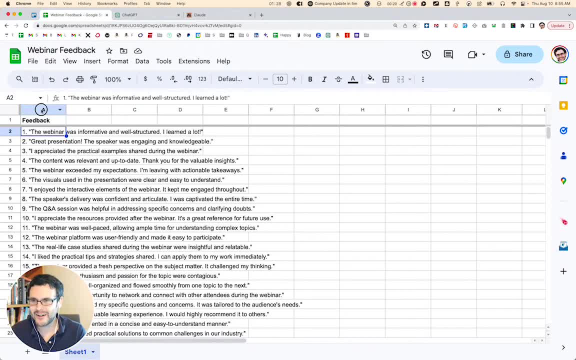 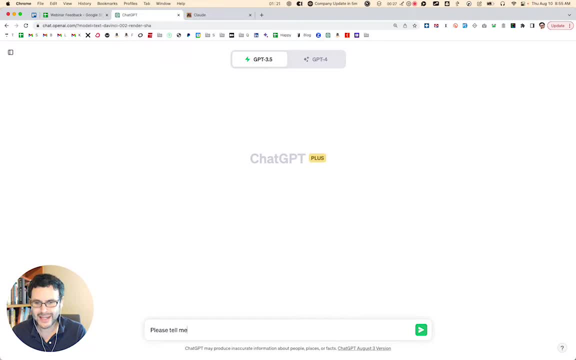 for AI to help Check this out. Go right over here to your feedback, grab it all, copy it, put it right into ChatGPT and say: please tell me the top three trends across this feedback And voila, you now have your own personal assistant that can figure out what's really. 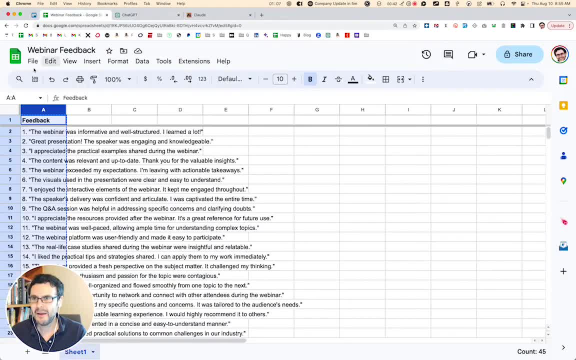 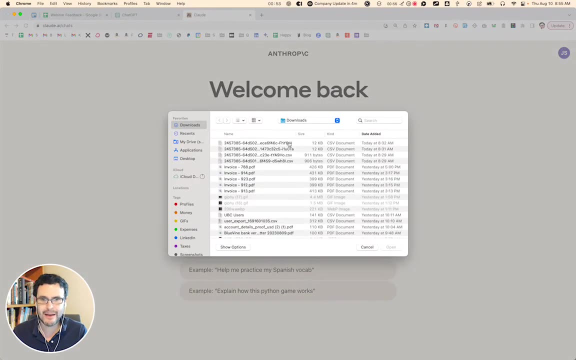 happening in that qualitative feedback. Or, better yet, maybe you come over here, you export that data to wherever you want. So, for example, download a CSV and then come over to clawai, a brand new tool in the space, And upload the file. And so you grab that file, you plug it in and say again: give me. 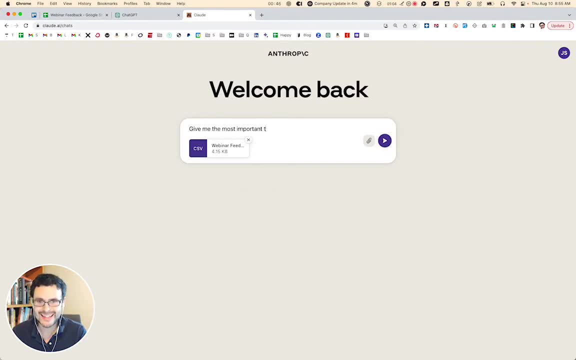 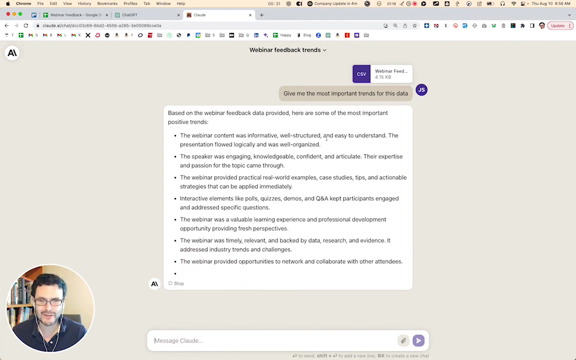 the most important trends for this data. It uploads the file, it scans it and here are the things that you really need to understand across hundreds or maybe even thousands of rows of open ended data. Again, your own personal research assistant at your fingertips all through the. power of AI. Hope you enjoy. Thank you so much for joining me today. I'll see you in the next video. 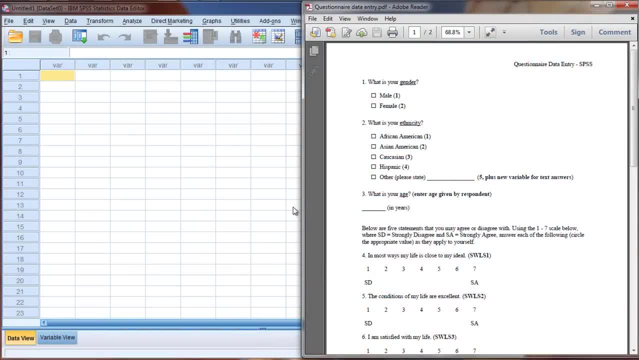 In this video, we'll take a look at how to enter questionnaire or survey data into SPSS, And this is something that a lot of people have questions with, so it's important to make sure when you're working with SPSS, in particular, when 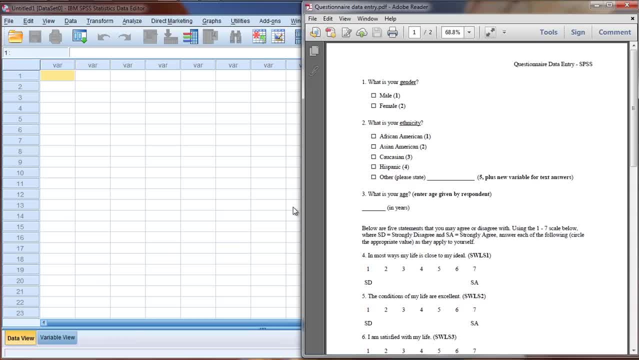 you're entering data from a survey that you know how to do. So let's go ahead and take a few moments to look at that. And here you see, on the right hand side of your screen, I have a questionnaire, a very short sample questionnaire that I want to enter into SPSS. So we're going. 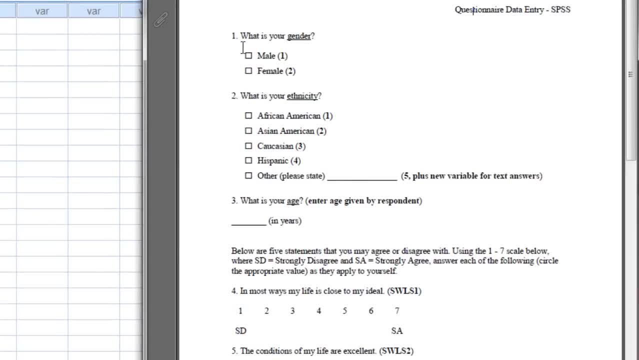 to create a data file, And in this questionnaire here I've made a few modifications. I've underlined some variable names here- and I'll talk about that more in a minute- And I also put numbers and parentheses to the right of these different names, And I'll also explain that as well.